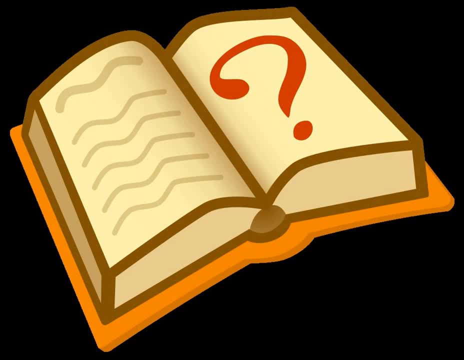 things that think. Rather than propose a single definition for ubiquitous computing and for these related terms, a taxonomy of properties for ubiquitous computing has been proposed, from which different kinds or flavors of ubiquitous systems and applications can be describedUbiquitous computing touches on a wide range of research topics, including distributed computing, mobile. 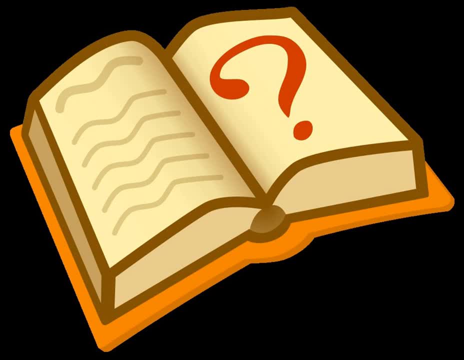 computing, location computing, mobile networking, context-aware computing, sensor networks, human-computer interaction and artificial intelligence. == Core concepts ==. At their core, all models of ubiquitous computing share a vision of small, inexpensive, robust, networked processing devices distributed at all scales throughout everyday life. 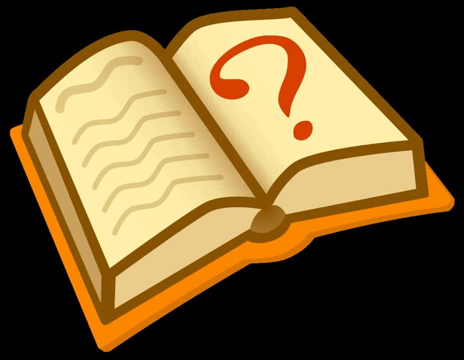 and generally turned to distinctly commonplace ends. For example, a domestic ubiquitous computing environment might interconnect lighting and environmental controls with personal biometric monitors woven into clothing so that illumination and heating conditions in a room might be modulated continuously and imperceptibly. Another common scenario posits refrigerators. 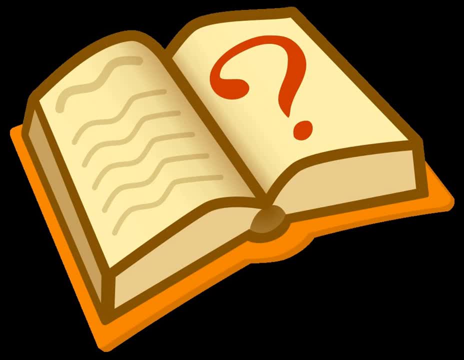 aware of their suitably tagged contents, able to both plan a variety of menus from the food actually on hand and warn users of stale or spoiled food. Ubiquitous computing presents challenges across computer science: in systems design and engineering, in systems modeling. 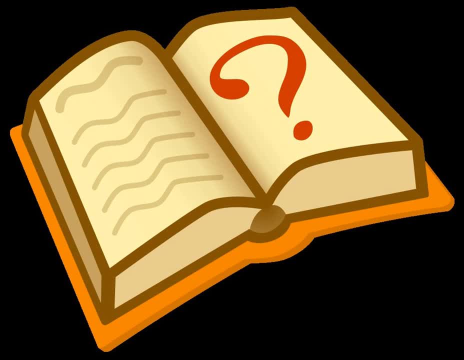 and in user interface design. Contemporary human-computer interaction models, whether command-line, menu-driven or GUI-based, are inappropriate and inadequate to the ubiquitous case. This suggests that the natural interaction paradigm appropriate to a fully robust, ubiquitous computing has yet to emerge. 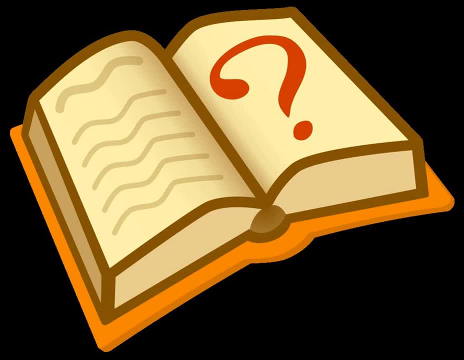 although there is also recognition in the field that in many ways we are already living in a ubicomp worldSee also the main article on natural user interfaces. Contemporary devices that lend some support to this latter idea include mobile phones, digital audio players, radio frequency identification tags, GPS and interactive. 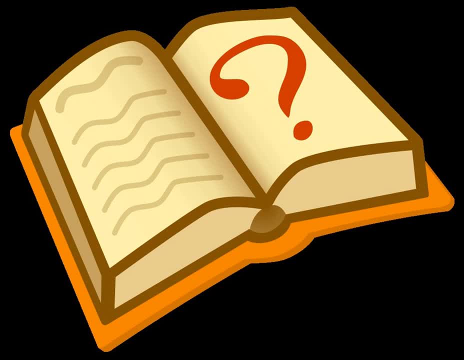 whiteboards. Mark Weiser proposed three basic forms for ubiquitous system devices: tabs, pads and boards. tabs- wearable centimeter-sized devices and USB这 номo which gives us active, batterian and sliding touch buttons. tabs- wearable centimeter-sized devices. pads- handheld decimetre-sized devices. 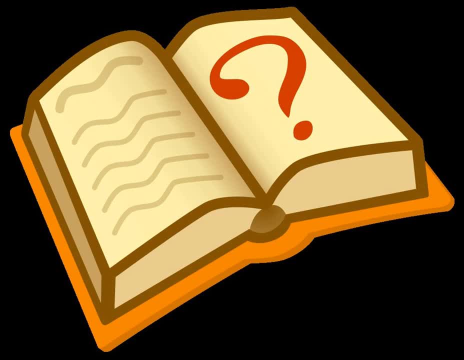 boards. meter-sized interactive display devicesThese three forms proposed by Weiser are characterized by being macro-sized, having a planar form and on incorporating visual output displays. Mark Weiser proposed three basic forms for ubiquitous system devices: tabs, wearable centimeter-sized devices and pads. interessante pieces of translate mechanical. 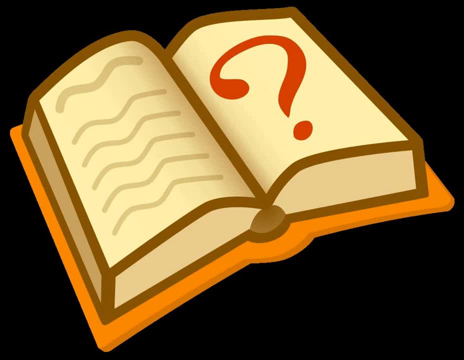 If we relax each of these three characteristics, we can expand this range into a much more diverse and potentially more useful range of ubiquitous computing devices. Hence, three additional forms for ubiquitous systems have been proposed: Dust miniaturized devices can be without visual output displays, eg. micro-electromechanical systems, MEMS ranging from nanometers through. 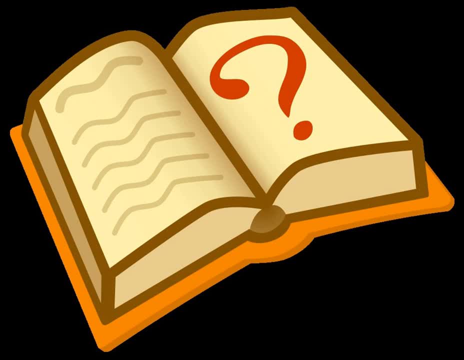 micrometers to millimeters. See also smart dust Skin fabrics based upon light emitting and conductive polymers. organic computer devices can be formed into more flexible non-planar display surfaces and products such as clothes and curtains: see OLED display. MEMS device can also be painted. 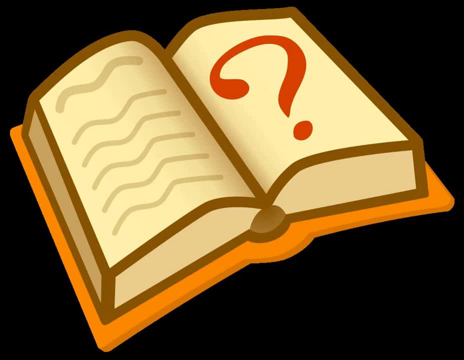 onto various surfaces so that a variety of physical world structures can act as networked surfaces of MEMS. Clay ensembles of MEMS can be formed into arbitrary three-dimensional shapes as artifacts resembling many different kinds of physical object. see also tangible interfaceIn his book The Rise. 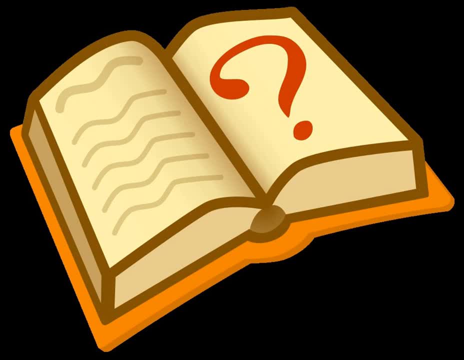 of the Network Society, Manuel Castells suggests that there is an ongoing shift from already decentralized stand-alone microcomputers and mainframes towards entirely pervasive computing. In his model of a pervasive computing system, Castells uses the example of the Internet as the start of a pervasive computing system. 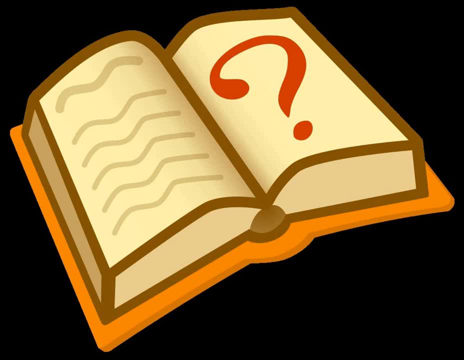 The logical progression from that paradigm is a system where that networking logic becomes applicable in every realm of daily activity, in every location and every context. Castells envisages a system where billions of miniature ubiquitous inter-communication devices will be spread worldwide like pigment in the wall paint. 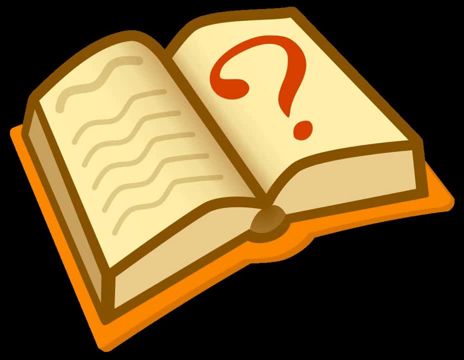 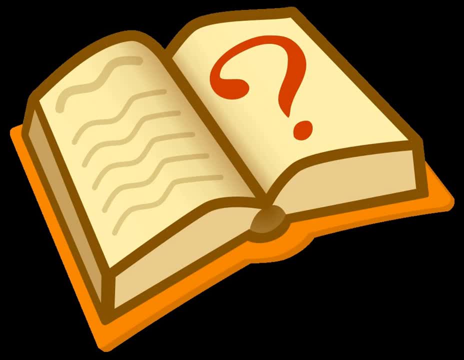 a single system. Tell us more about the system. 1. Steps for bitcoin. 2. Energykhana Background Memory Wallpapers. manage reliability of the resources. == History ==. Mark Weiser coined the phrase "ubiquitous computing" around 1988, during his tenure as chief technologist of the Xerox. 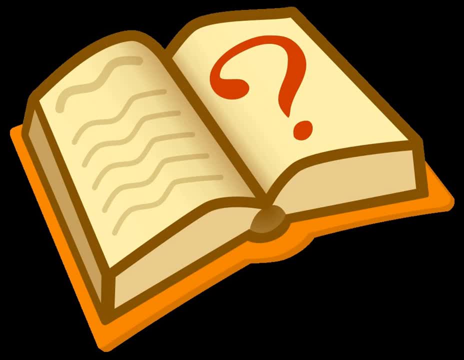 Palo Alto Research Center, Both alone and with Park director and chief scientist John Seeley. Brown Weiser wrote some of the earliest papers on the subject, largely defining it and sketching out its major concerns: ====. Recognizing the effects of extending processing power ====. 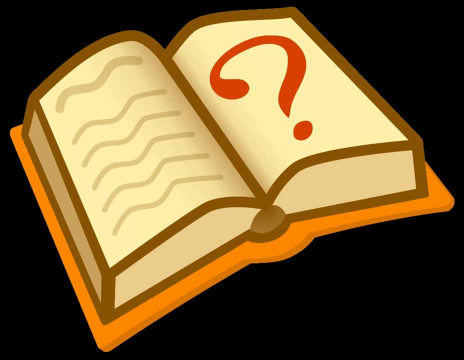 Recognizing that the extension of processing power into everyday scenarios would necessitate understandings of social, cultural and psychological phenomena. beyond its proper ambit, Weiser was influenced by many fields outside computer science, including philosophy, phenomenology, anthropology, psychology, physics and mathematics. 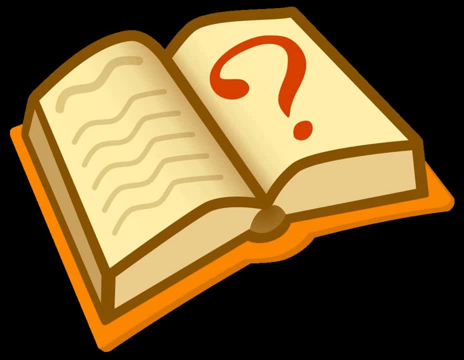 He was also inspired by the concept of postmodernism, sociology of science and feminist criticism. He was explicit about the humanistic origins of the ''invisible ideal'' in postmodernist thought, referencing as well the ironically dystopian Philip K Dick novel Ubik. 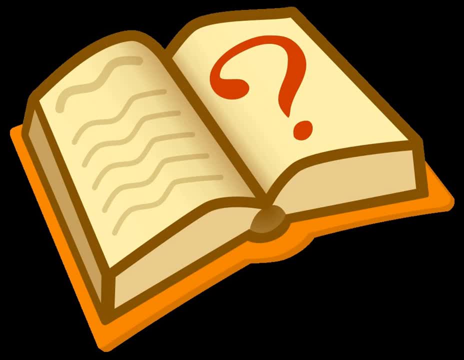 Andy Hopper from Cambridge University, UK, proposed and demonstrated the concept of ''teleporting'', where applications follow the user wherever he she moves. Roy Wont, while a researcher and student working under Andy Hopper at Cambridge University, worked on the ''Active Badge System'', which is an advanced location computing system. 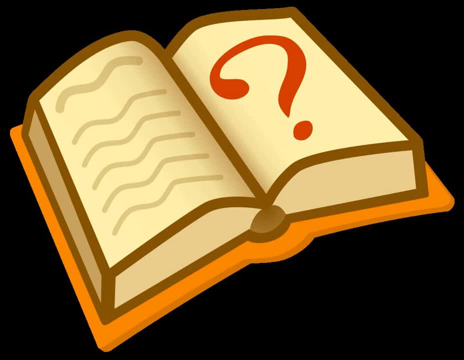 where personal mobility that is merged with computing. Bill Shillett also did some earlier work in this topic and participated in the Early Mobile Computing Workshop held in Santa Cruz in 1996.. Ken Sakamura of the University of Tokyo, Japan, leads the Ubiquitous Networking Laboratory. 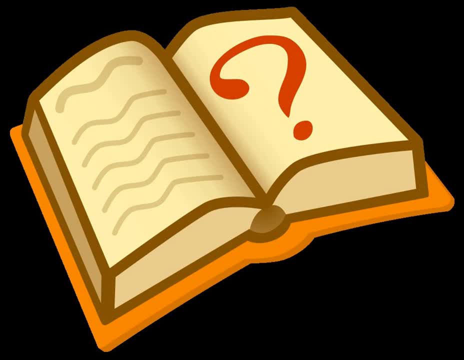 Tokyo, as well as the T-Engine Forum. The joint goal of the T-Engine Forum is to develop a new technology that can be used in the future. The goal of the T-Engine Forum is to develop a new technology that can be used in the future. 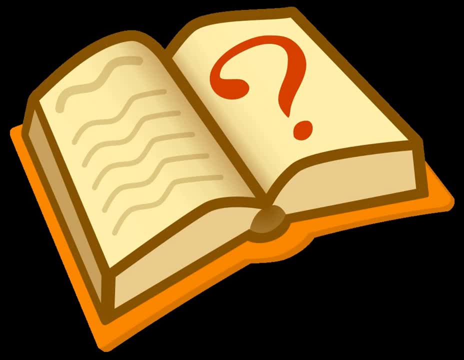 The goal of Sakamura's Ubiquitous Networking Specification and the T-Engine Forum is to enable any everyday device to broadcast and receive informationMIT has also contributed significant research in this field, notably things that Think, Consortium directed by Hiroshi Ishii, Joseph A Paradiso and Rosalind Picard at the Media Lab and the CSAIL effort. 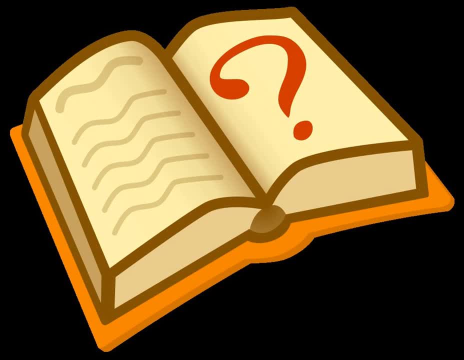 known as Project Oxygen. Other major contributors include University of Washington's Ubicomp Lab, directed by Shwetak Patel, Georgia Tech's College of Computing. Cornell University's People Aware Computing Lab, NYU's Interactive Telecommunications Program. UC Irvine's Department of Informatics. 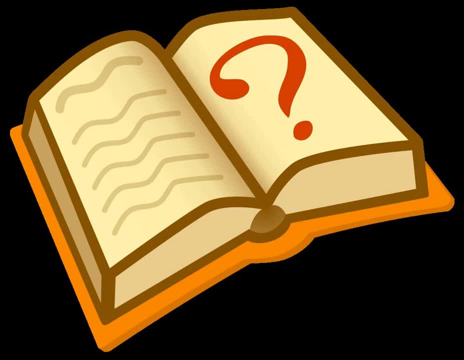 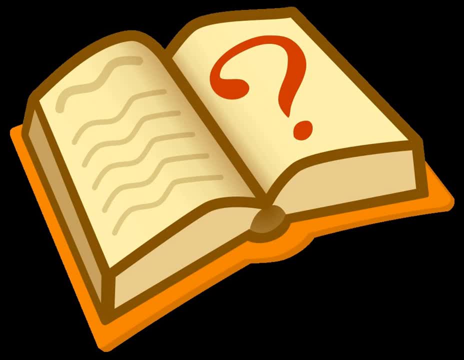 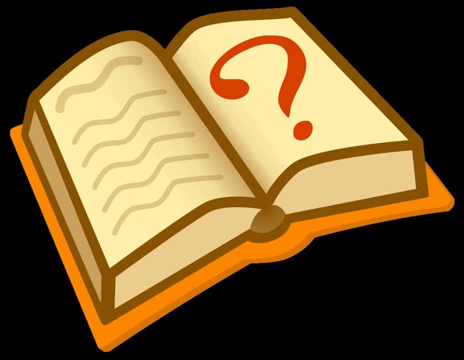 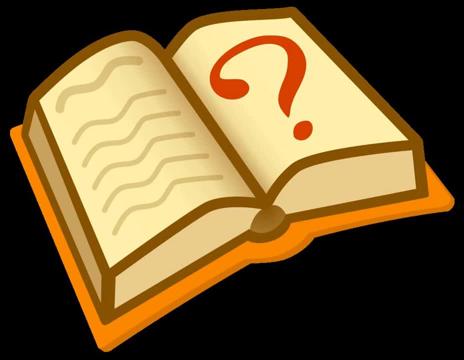 ==== Webinar. ==== fusion of mobile phones, Many of mobile phones supporting high-speed data transmission, video services and mobile devices with powerful computational ability, Although these mobile devices are not necessarily manifestations of ubiquitous computing, there are examples such as Japan's Yayorozu 8 million gods project, in which mobile devices 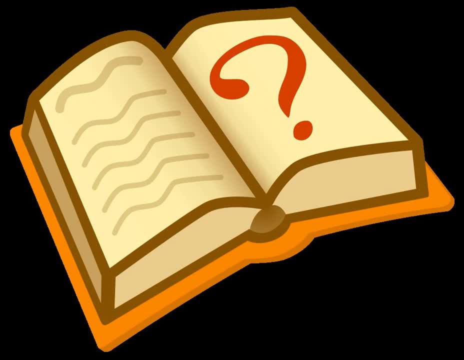 coupled with radio frequency identification tags, demonstrate that ubiquitous computing is already present in some formAmbient Devices has produced an orb, a dashboard and a weather beacon. These decorative devices receive data from a wireless network and report current events such as stock prices and the weather, like the NABAS tag. produced by Violet Snowden. The Australian futurist Mark Pess has produced a highly configurable 5-2 LED lamp-enabled lamp which uses Wi-Fi, named Moore's Cloud after Moore's LawThe Unified Computer Intelligence Corporation has launched a device called UBI, the ubiquitous 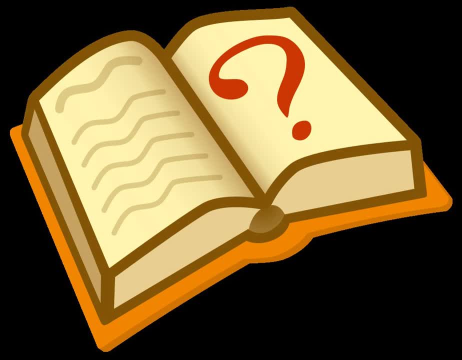 computer that is designed to allow voice interaction with the home and provide constant access to informationUbiquitous computing research has focused on building an environment in which computers allow humans to focus attention on select aspects of the environment and operate in supervisory and policy-making roles. Ubiquitous computing emphasizes the creation of a human 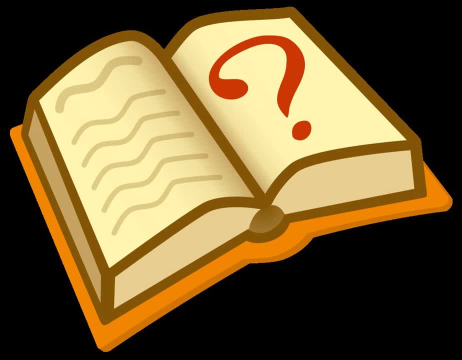 computer interface that can interact with the environment and the environment itself. The computer interface is designed to support and interpret and support a user's intentions. For example, MIT's Project Oxygen seeks to create a system in which computation is as pervasive as air. In the future, computation will be human-centered. It will be freely. 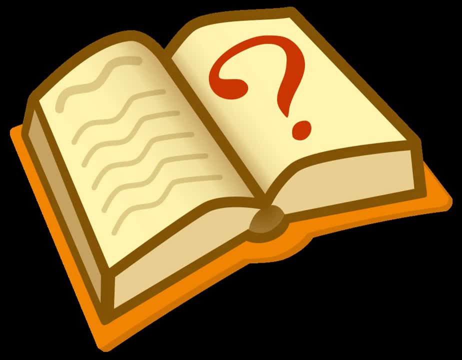 available everywhere, like batteries and power sockets or oxygen in the air we breathe. We will not need to carry our own devices around with us. Instead, configurable generic devices, either handheld or embedded in the environment, will be able to communicate with each other and communicate with each other. We will not need to carry our own devices. 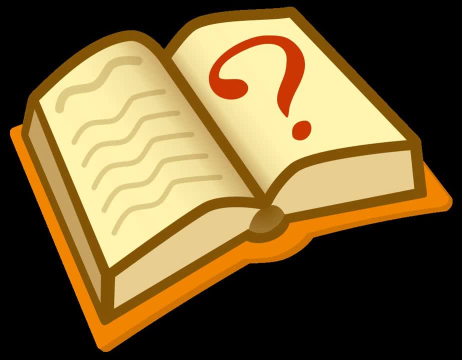 around with us. Instead, configurable generic devices, either handheld or embedded in the environment, will bring computation to us whenever we need it and wherever we might be. As we interact with these anonymous devices, they will adopt our information personalities. They will respect our desires for privacy and security. We won't have to 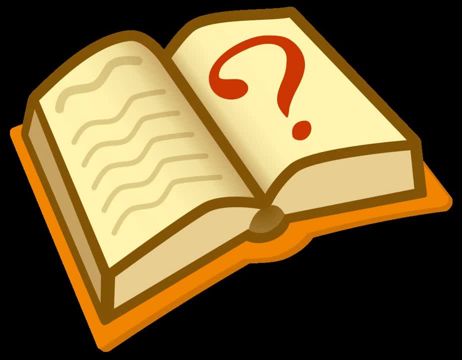 type, click or learn new computer jargon. Instead, we'll communicate naturally, using speech and gestures that describe our intent. This is a fundamental transition that does not seek to escape the physical and the emotional. We will not need to carry our own devices. 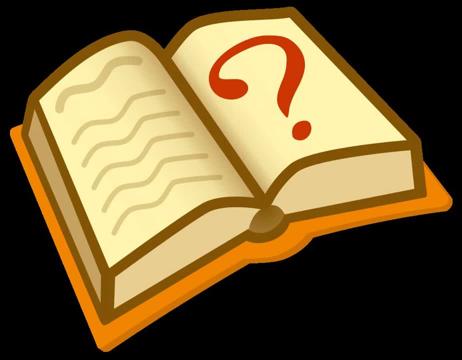 around with us. Instead, we'll interact with these devices. They will recognise our intentions, values and appropriate abstinence, and we'll be able to record our actions. in fact, The world is more than us. When we're children, we can laugh andCI' Only then. 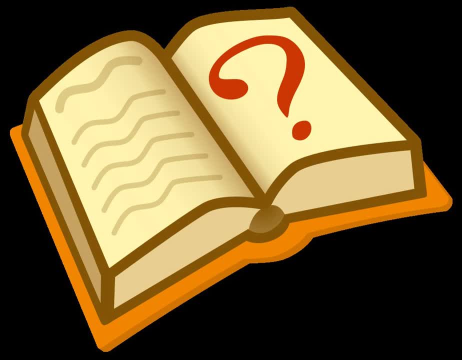 can you forget everything, So make these memories a habit. == Barrier ==. == Values ==. often cited criticism of ubiquitous computing, Ubicomp, and may be the greatest barrier to its long-term successAn article by Linda Little and Pam Briggs on this privacy issue states that 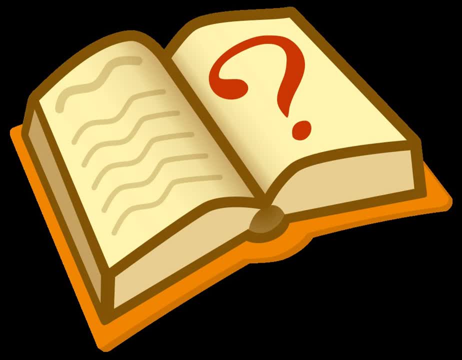 these are the kinds of privacy principles that have been established by the industry, but over the past two years we have been trying to understand whether such principles reflect the concerns of the ordinary citizen. Some of the key research questions we have been addressing are: 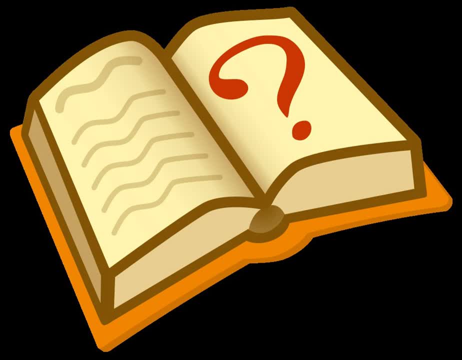 what are users' key concerns regarding privacy management in a ubiquitous context, and do they reflect expert privacy principles? Do these concerns vary as a function of context? Will users have enough confidence in privacy management procedures to hand over management and administration of their privacy preferences? Modahari et al 2007, argue people do not have a complete 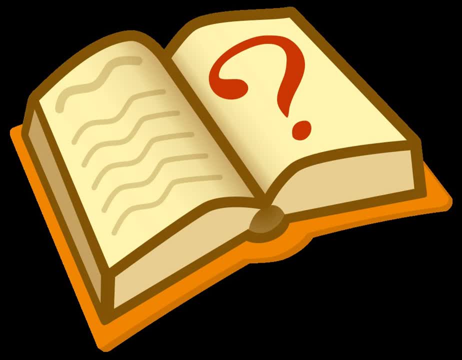 understanding of the threats to their privacy. While users of Ubicomp systems are aware of inappropriate privacy, they are not aware of the threats to their privacy, use of their personal information, legal obligations and inadequate security. they are less aware of setting preferences for who has access and any social inferences that can. 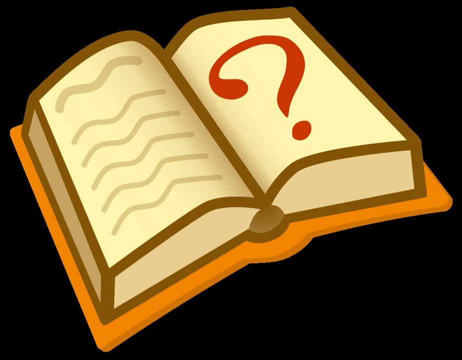 be made by observations by other people. They further argue a holistic approach is needed as traditional approaches and current investigations are not enough to address privacy threats in ubiquitous computing Recognizing, in line with a number of other researchers- Harper and Singleton 2001,, Payne et al 2007,. 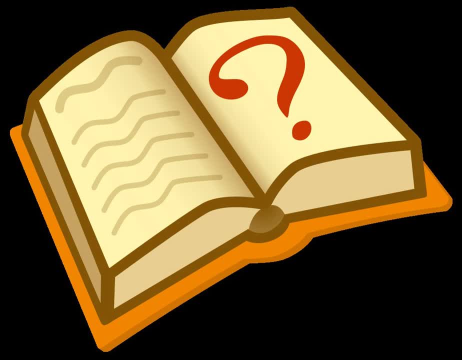 that privacy concerns are likely to be highly situation-dependent. we have developed a method of inquiry which displays a rich context to the user in order to elicit more detailed information about those privacy factors that underpin our acceptance of ubiquitous computingPublic policy problems are often preceded by long shadows, long trains of activity emerging slowly over decades. 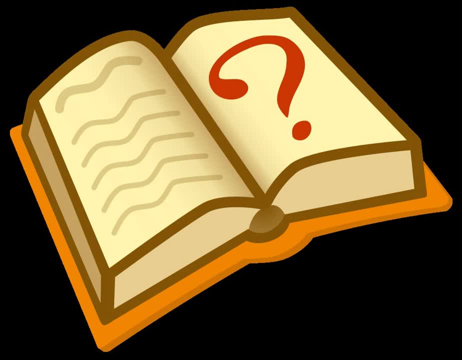 or even the course of a century. There is a need for a long-term view to guide policy decision-making, as this will affect the future of privacy. This will assist in identifying long-term problems or opportunities related to the ubiquitous computing environment. This information can reduce uncertainty and guide the decisions of both policy makers and 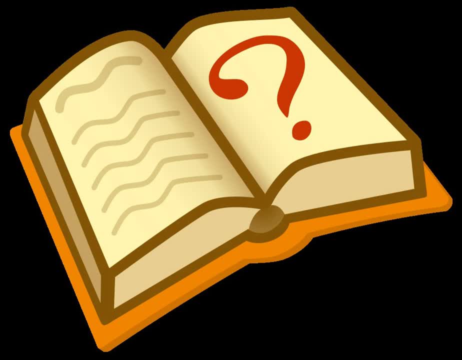 those directly involved in system development. Wedemeyer et al 2001.. One important consideration is the degree to which different opinions form around a single problem. Some issues may have strong consensus about their importance, even if there are great differences in opinion regarding.